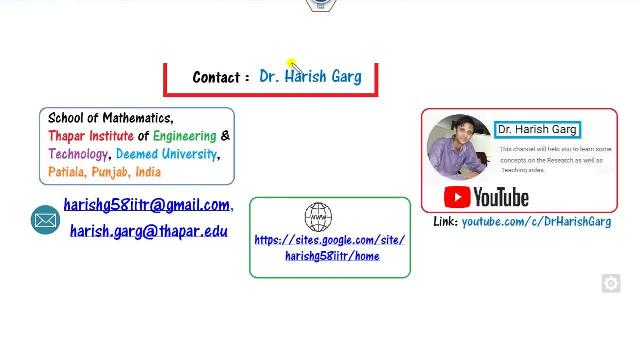 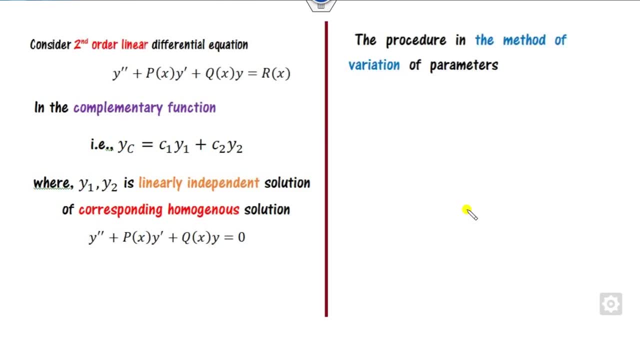 method in this video to explain this: Myself, Dr Gurk, working in the school of mathematics, Thapar Institute. You can simply follow this link for finding this: various videos on the mathematics subject. So as we know that there is a complementary solution is written by here: c1, y1 plus c2, y2, where c, y1 and y2 are the 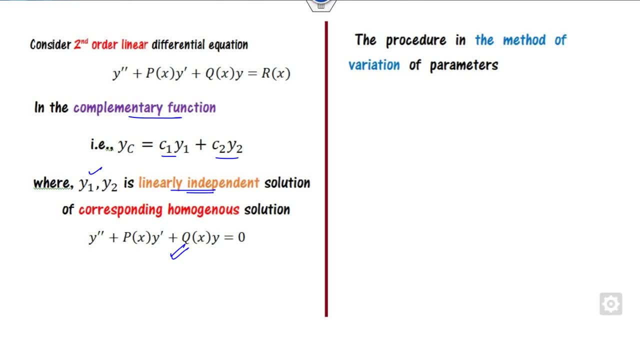 linear, independent solution of homogeneous part. Now, what is the procedure of the variation of parameters? So you can see that here the c1 and c2 are my constants. So you remember that whenever you are talking about the complementary functions, here c1 and c2 are the constants. But here, in this method, instead of 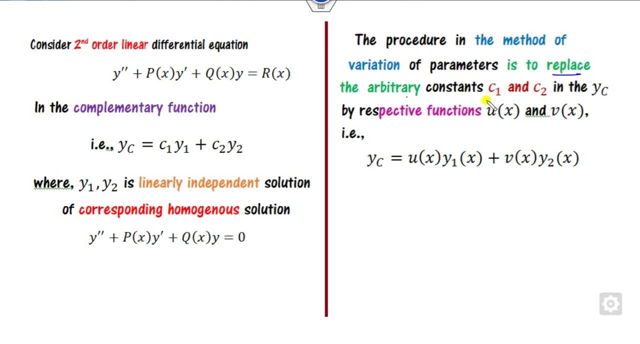 the taken as a constant. we will replace this arbitrary constant c1 and c2 with the respective functions of the x and y. I call as the u and the v like here. This is: I replace constant with respect to the function. Then our target is to identify this u and v. That is our target Once. 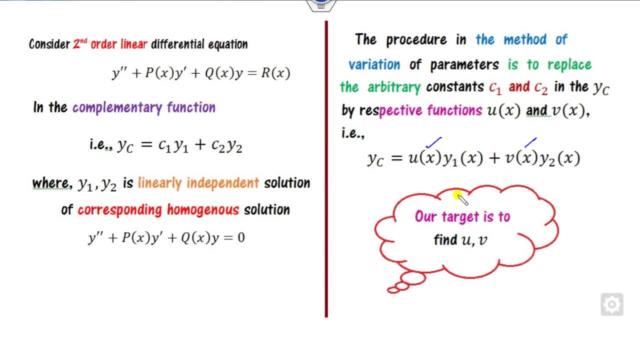 it is a function of the x and x here. then what is the value of the u and the v? So this is the u and v. How you find that. So our target is to find the value of u and v so that the resulting 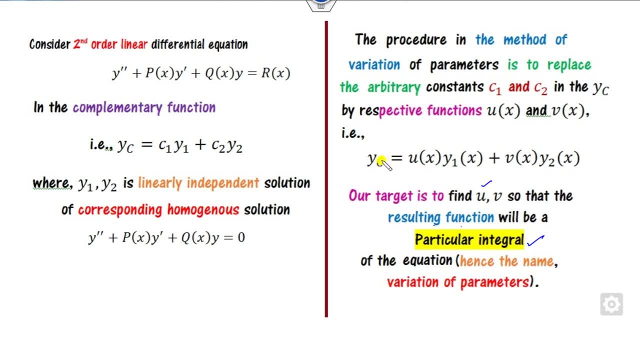 function will be the particular integral. So I call this yc as a yp. when you consider here And now, you can see why it is called as the variation of parameter, because this u and v are vary with respect to the x are there. So that's why, hence, the name is called as the. 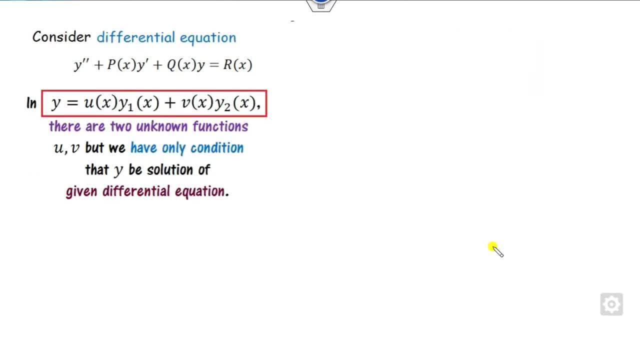 variation of the parameter. Now how you can solve them Once we consider this as a here, the two unknown parameter, u and v. So once and we know this is the one condition are there, So we can find the, we are free to impose the second condition because there are the two unknown. 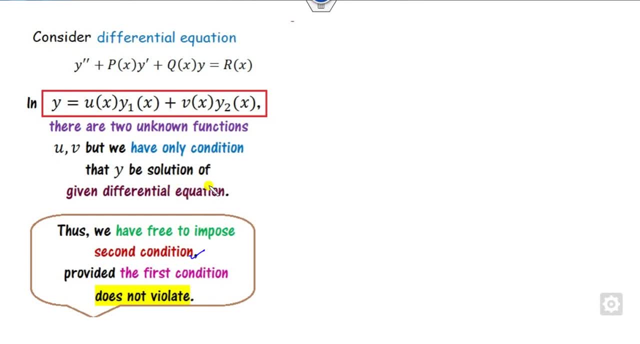 parameters. Our target is to find the values of the u and v. So what you can do, That's very simple. You can take us here, You can substitute this value here. For that you need to calculate y dash and y double dash. as here You can see, I can take as a y dash is as a product rule. 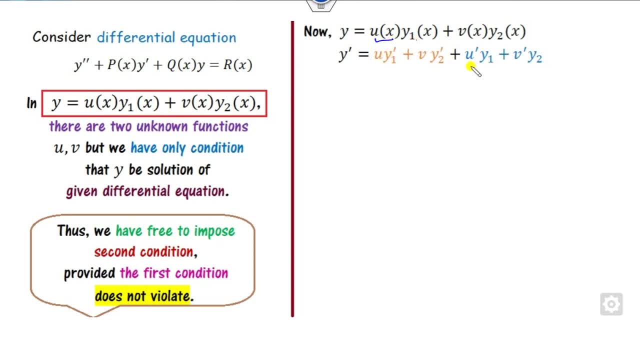 There is a first function derivative of second, and so on. me now what is the condition imposed on them? so i will consider this part as a zero. you can see here why: because u and v are taken from the constant part c1 and c2. if i consider u as a. 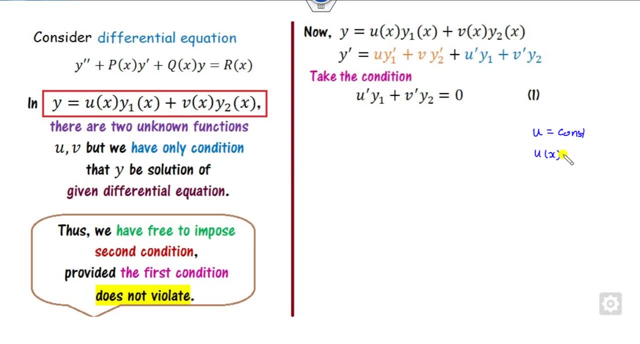 constant. what will happen if i consider as a u of x is 4? so definitely this part will be a non-zero, this part will be a zero. so it means my condition is taken as of here. second condition is: so once you substitute this value here, so y dash will be by this. now, similarly, you can find the y double. 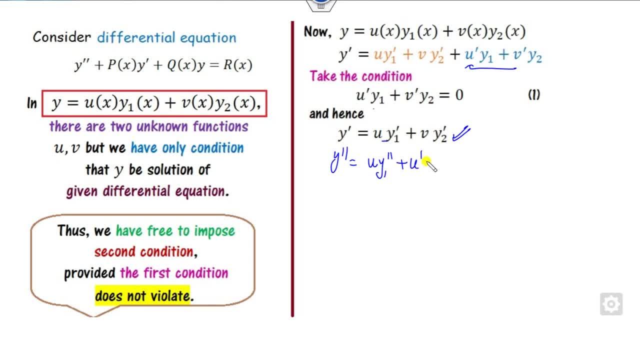 dash again. you can use as a product rule, so you can taken as of this and so on. so you can get here, substitute these two values in the given differential equation. you will get here. now you can equate. the pairs are there, you can see this, the u and so on. what is there? this is nothing. 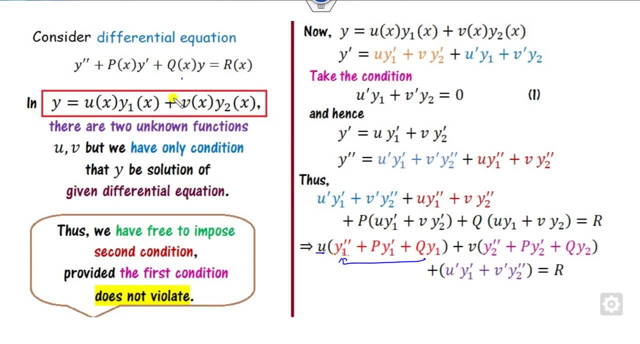 but the solutions of the y1, that is the y1, satisfied here. what is the y1? y1 is the solution of the homogeneous part. so what is the homogeneous part? are there? that is here. this is nothing. this is my zero. this is my zero. this is my zero. homogeneous part. this is my homogeneous part. 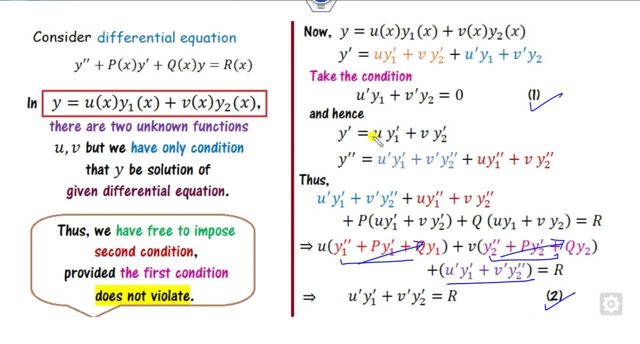 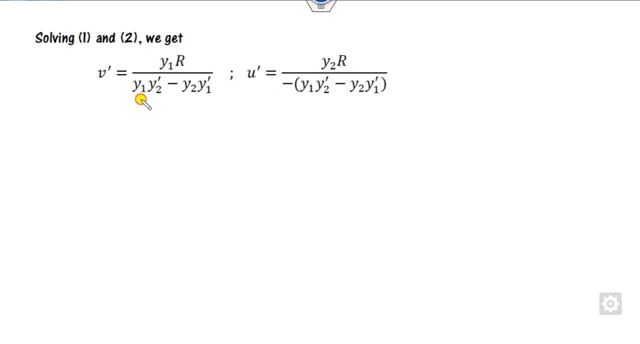 so that part is there. now you can solve this equation for 1 and 2. you can find the value of the u dash and v dash as here. once you will get here you can also you can see what is that denominator part are there. i can easily write as a wrong scale, that is, a y1 and y2 are given to you. 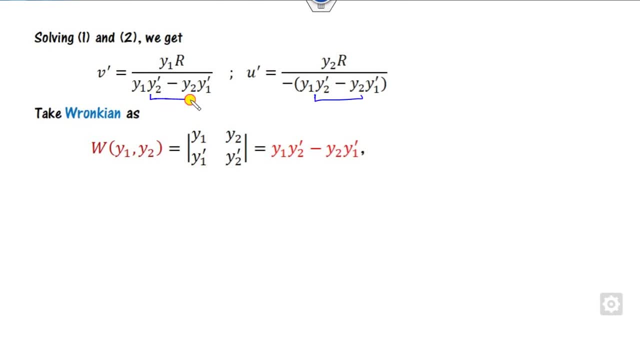 you can take as here. so what is that? this is nothing but w. this is nothing but w. so i can write here as of this. i can integrate on both side. so what will happen? this is nothing but my v. this is y1, r, w and dxr. 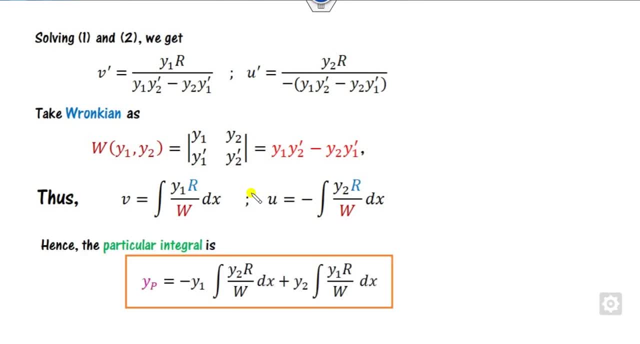 so this is the. once you will find the u and v, you can substitute this value, so you will get the particular integral here. you can also remember this in a very simple manner. you can see: this is y1, then it's a y2, first value. start from the negative, positive, negative positive and so on. 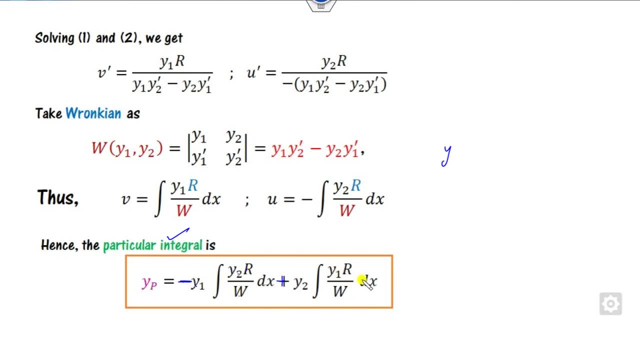 so minus y1, y2 and y3 and so on. so you can write here: as of this i can integrate on both side. so y2, r by w and so on in journal you can write. this is in summary, this is for the two variable. but if 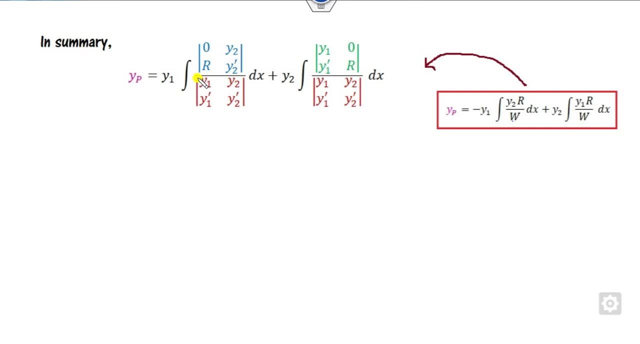 it has a three variable how you can write them. i can replace wrong Im. stories is written like this way: now, if you are written on the y1, these two things also have smaller- then the zero r is replaced on this first side. if you write on the second part, then you have to. 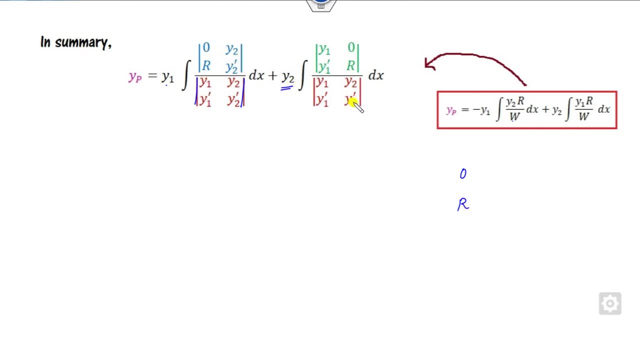 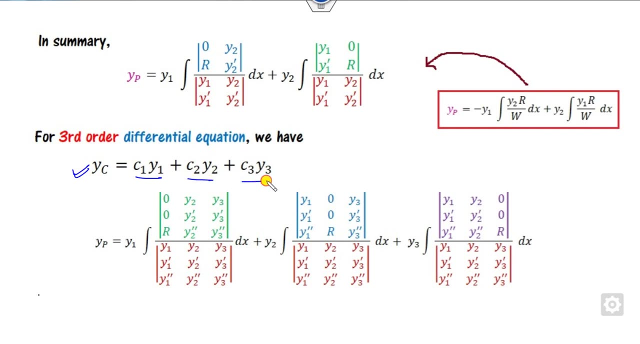 replace zero r on here. for example, if you have the three third ordered there, then you have to. x was right. how you can find the yc? you have to write it, because that sanders. so it is even if two choose from three order. we have to make it correct. then you have to e or c and u are. 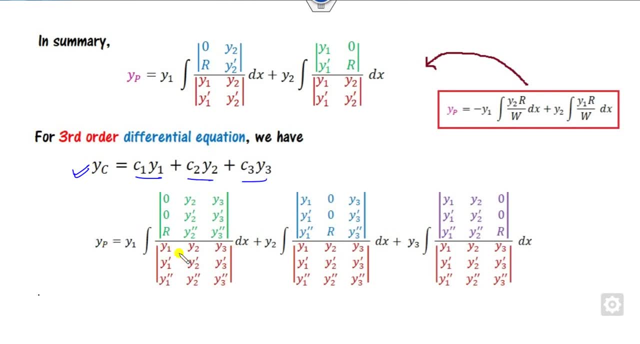 to be replaced. so u and c are actually same value. we have to go to one of these interior Кall a- and a- and they are not. is what is it? number three and n and N is a common space- can find the yc. you have to write the wrong scale of this: y1, y2, y3, determinant, second derivative. 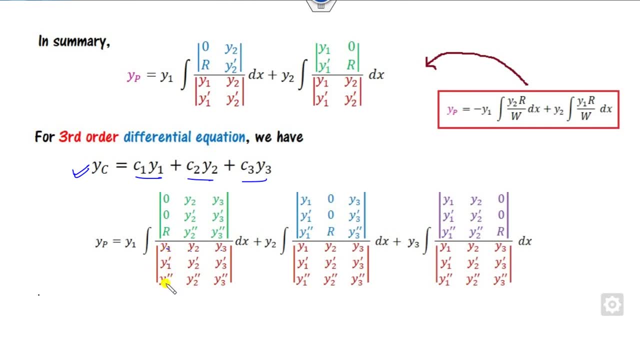 then what is the first part is you have to replace this as a 0 0 r. you can see 0 0 r, while the others are same. for the second part, i have to replace as a 0 0 r for this. for the third part, i have to. 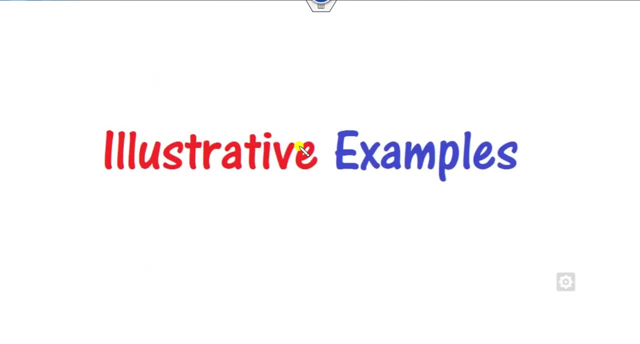 replace, as here now, in order to explain how you can solve them. we will see these four examples in this part. these four examples we will see, so let's start with the first one. so, since it is a secant of x, so your first target is to compute yc and yp. how you can compute the yc, as we discussed. 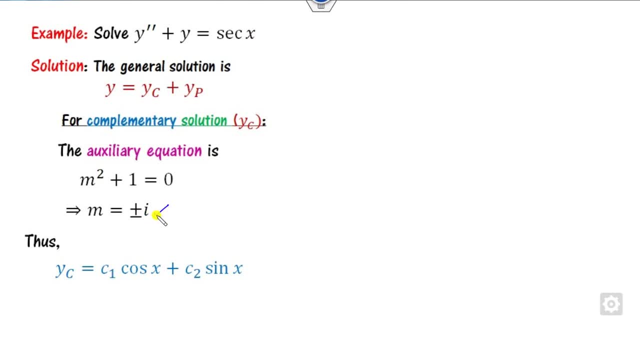 that you can consider auxiliary equations. you can see this is a plus minus iota. so therefore, here now. this is my y1, this is my y2. once you get the y1 and y2, you can compute this as a here, or you can also consider this as a determinant of this. but there is no need of them, since it is a. 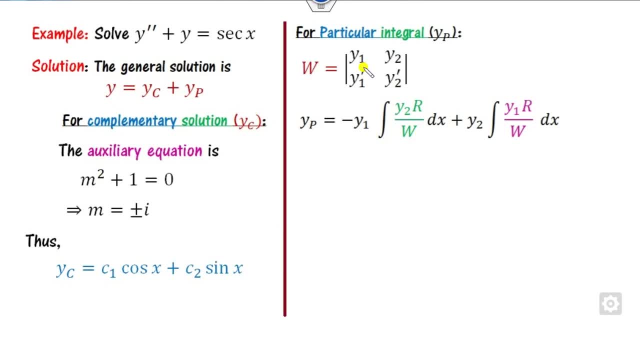 two variable. so first target is to find the value of the w here. so what is the y1? is this i consider as a y1, this as i consider as the y2, so i can substitute- here you will get the wrong skin- as a 1, so you can substitute. the value of y1 is nothing but my cos. 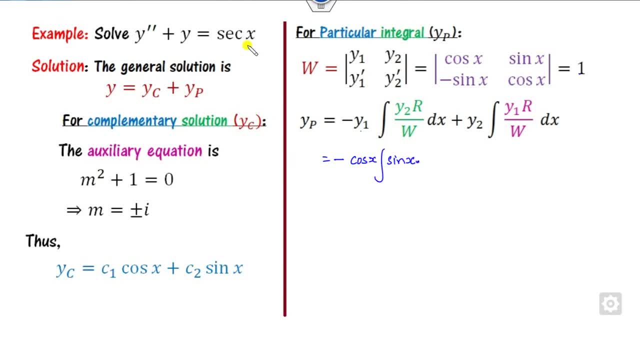 x. what is the y2 is nothing but my sine x. what is the r is my right hand side. this is secant of x. what is the w is my 1 plus of thin, and so on. you will get here. what is that? this is sine upon cos. 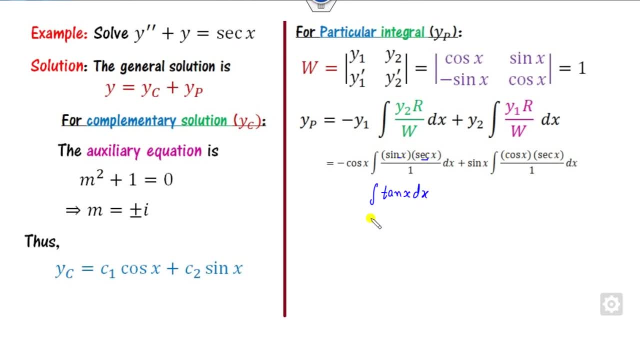 that is the integration of the tan x. so all of you know that. what is the integration of the tan x? this is nothing but my log of cos x. what is that? this is nothing but my 1. so integration of 1 is my x. now, integration of the tan x is nothing but my minus of minus plus. so this is nothing but my. 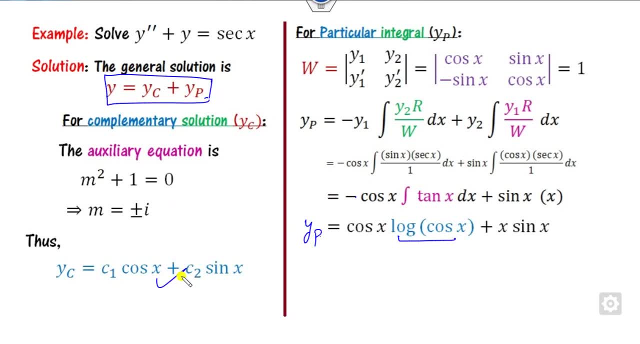 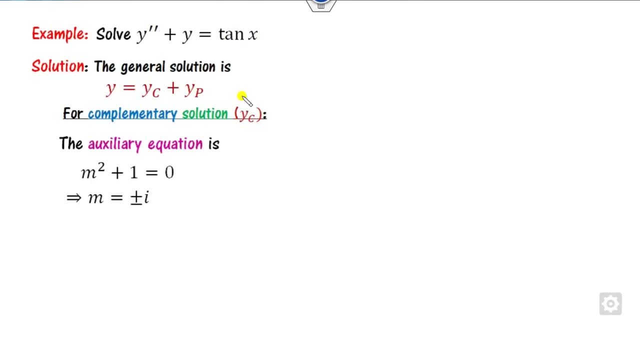 yp. so therefore, you can substitute the value here. this is the yc, this is my yp. you will get the general solution here. similarly, we can quickly move on the second example. you can firstly solve this complementary part and you will get the yc as here now. this is my y1, this is my y2. 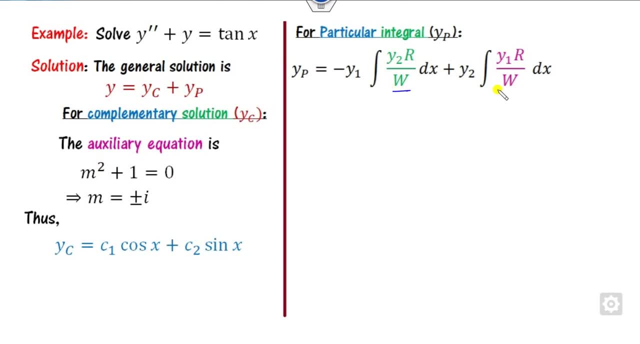 you can find the particular integral by using here. you can find the value of the w. that's again wrong skin. as a 1 you can substitute here: y1 is nothing but my cos, x and so on. you can see this is the sine. is my y2, r is nothing but my tan. so if you solve them, this is sine square upon cos. 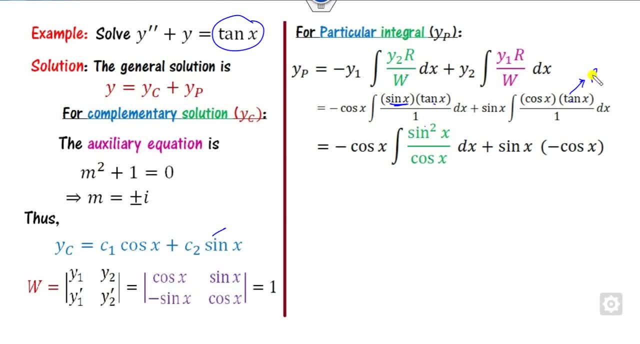 this is sine upon cos. this is nothing but my integration of sine x. what is the integration of the sine x? this is nothing but my cos x. how you can solve them? you can easily solve them by using here as cos. either you can take as a cos x is y, or else you can. 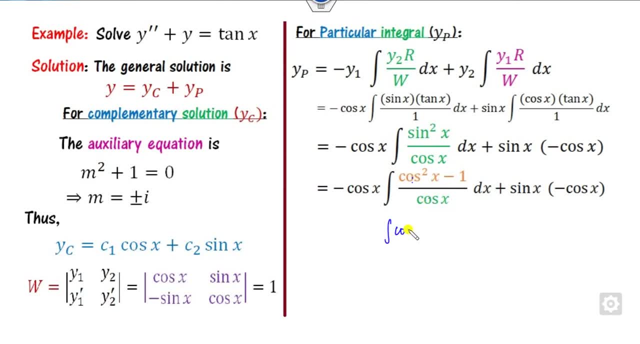 simply take an s here. now what is that? this is nothing but my cos of x. dx minus 1 upon cos is nothing but my secant x of dx. so what is the integration of the cos? x is nothing, but my sine secant is nothing but here. so this is my yp. you can substitute this yp here. you will get the. 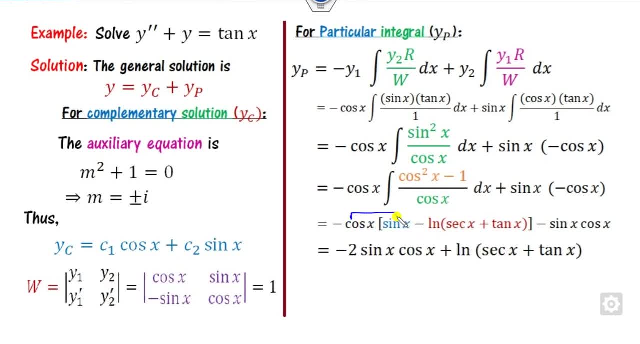 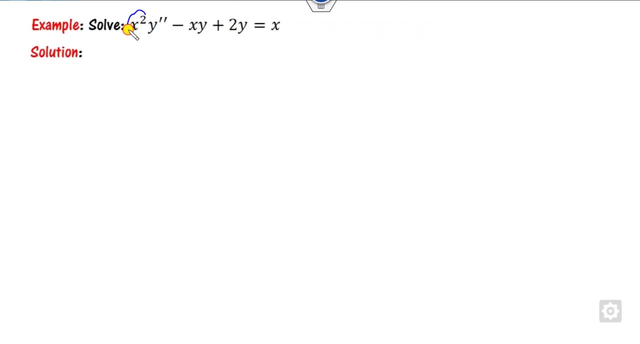 solution as of this or otherwise. you can more simplify. this is cos x sine x. this is cos x sine x. it will be the 2 sine x cos x, or you can also write this as of sine of 2x. so the general solution is my. here you can see. one more example are there. now you can see. this is: 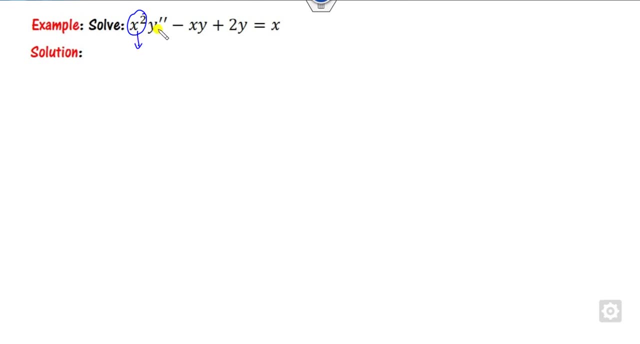 a, not a constant. the, the coefficient of the y double dash is not a constant, so we will firstly convert this into the constant coefficients. if you closely look about that, which form is there x square y double dash? this is the cauchy eiler equation. so once this, then 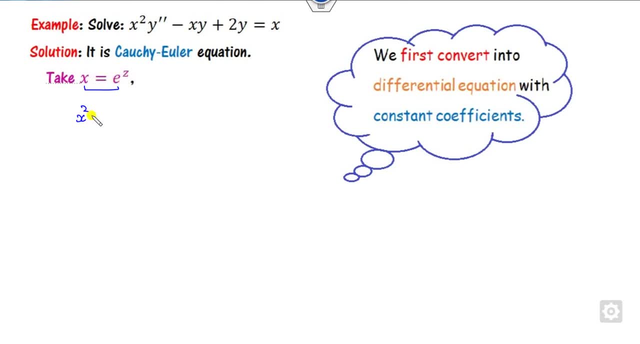 it's cauchy eiler. you have to use x as eris power z. so what is the value of this? this is nothing but my d square y upon dz square minus of here. and what is the value of the xy dash is this, is the. 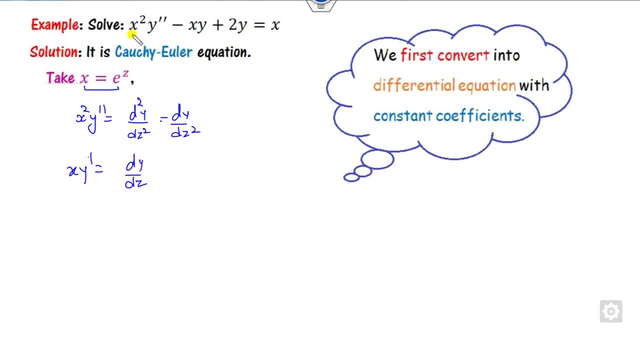 first derivative. so you have to take a like here. substitute these two values in here. this- sorry, this is a y dash. this is a y dash- is a typing error. so this is my y dash. you can substitute the value here. you will get this one. now, this is the constant coefficients. you can find the. 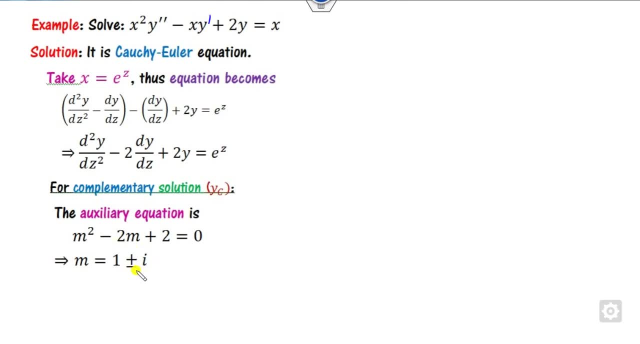 equation as of here. this is plus minus 1 plus minus iota, so this is alpha plus minus iota form. you can find the auxiliary equation as here now, since it is in the form of the z, now you can find this particular integral of this. this is the w, so what is the y one? so y one is my if you multiply. 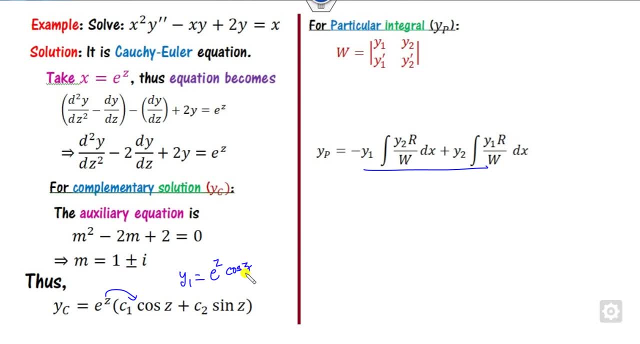 them. it will be my e eris power z, cos of z. and what is the y2 is my e rest power z, sine of z. so you can substitute the value here. you can see, this is the e. and here you can solve them. you will get this expression. you can substitute the value here: this is e rest. 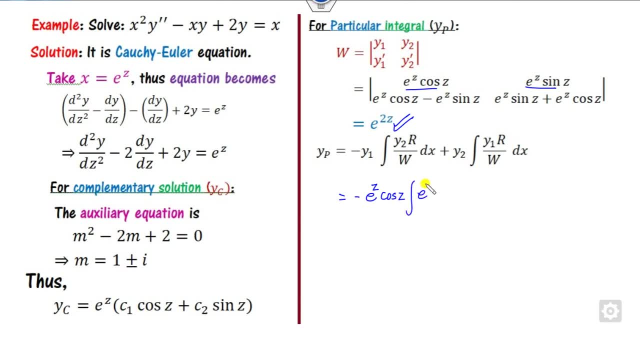 power z cos of z. what is the y2? is my e rest power z of sine z. what is the r? now, this is not the r, since you convert this value in terms of the z. so this upon y w is my here now, instead of the x. 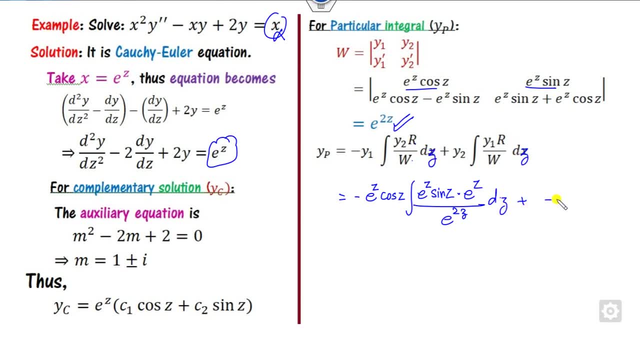 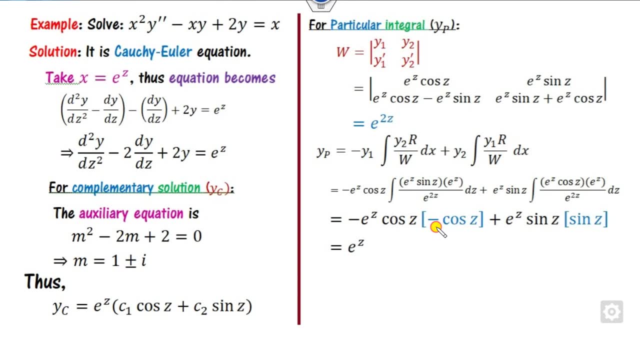 here as a z is there because all the transformation are there. now you can see this will be cancelled. integration of the sine z is nothing but my cos z is there. similarly for here now, after the simplify, you can see: cos square plus sine square is 1 here now, what is the general solution here? yc plus yp. 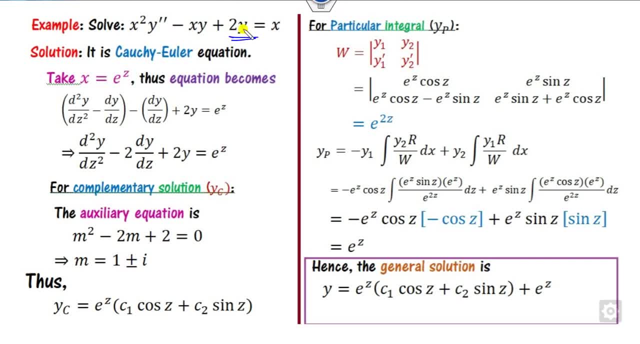 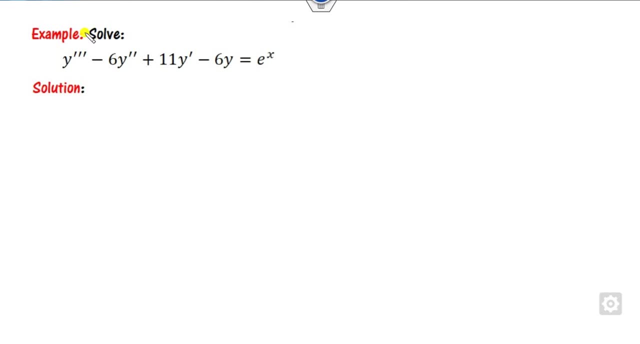 here, but our given equation in the terms of the x. so what is the value of the ez is nothing but my x. what is the z is my. you can find the value of the z from here. this is nothing but my log fx. you can substitute is the right answer. look at the third one is last question. is there now? 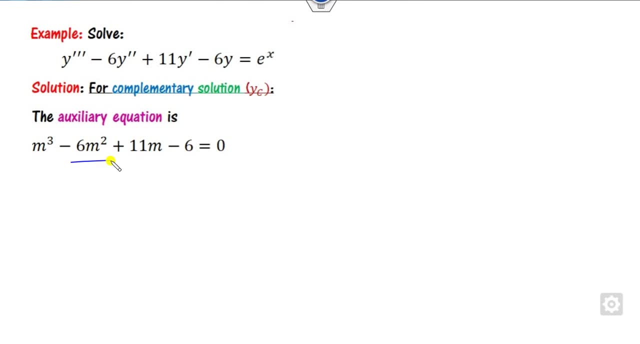 here is a y triple dash, so what you can do is you can write the auxiliary equation here. you can clearly see that n is equal to 1 is the root of this equation. so i can write like this way: what is the root of this? this is the 2 and 3, so here. so therefore my yc is there now this. 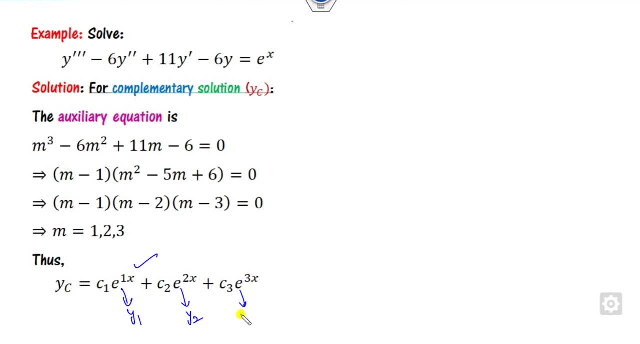 is considered as a y1, this is considered as a y2, this is considered as a y3. so how you can define the yp is now. you can see that here. that is a wronskian, this is a denominator, is wronskian. the first part is replaced by 0. 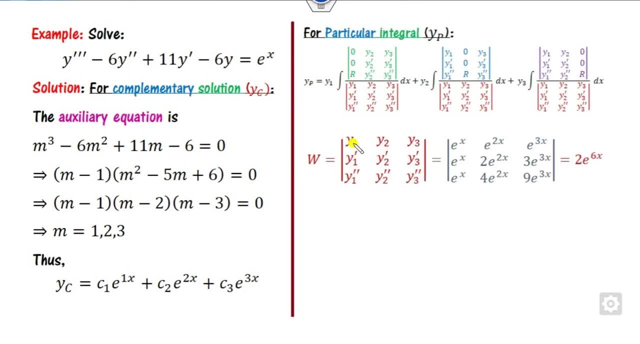 0r second part is 0, 0 and so on. so i can take it as a. y is e raised power, z, 2x and 3? i can find the derivatives and you can solve this as a determinant. you can easily solve them. e raised power, x, common. 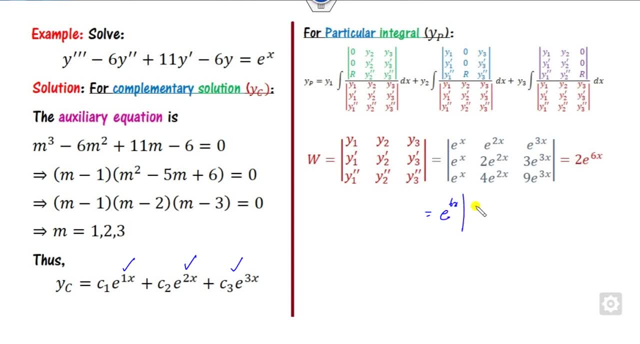 from here. e raised power 2x, so e raised power 6x common from this. so this is 1: 1. 1. 1, 2, 4. 1, 3, 9. now you can easily expand them. you will get here. similarly, you can solve this value. this is 0: 0. 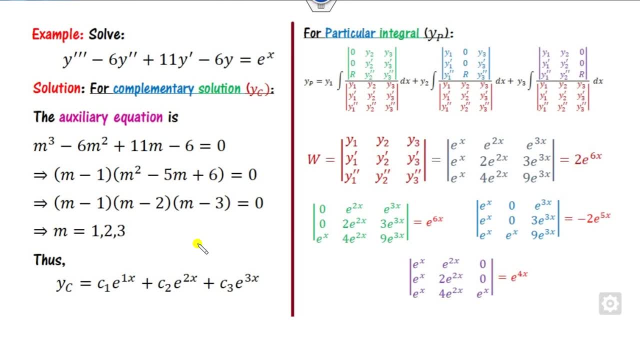 r is my e raised power x, y2 is my e raised power 2x. so you can see that similarly for this part- this blue part is here, this purple part is my here and green part is there. once you will get the expressions are there, you can substitute the value. 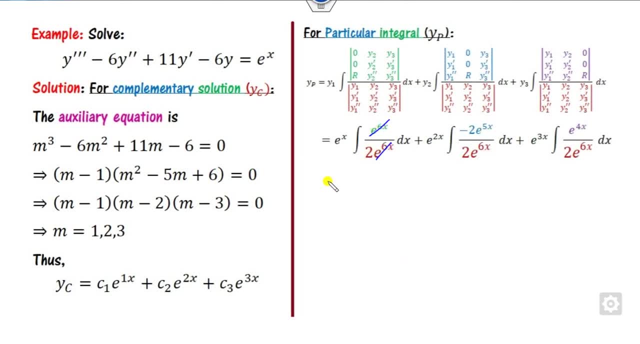 here. you will get this one so you can see. this value is half. this is nothing, but my x by 2. this value is nothing, but my 2 will be cancelled out. minus is outside. so what is that? e raised power minus of 1x divided by minus 1, it will be e raised power 3x by. 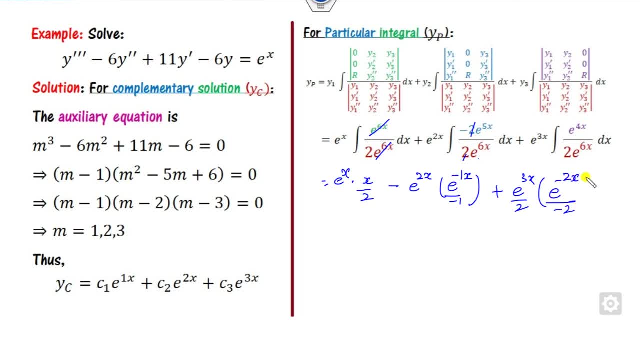 2 outside e raised power. minus of 2x divided by minus of 2 is the right answer. so you, after the simplify, you will get this. so what is the right answer is yc plus yp is here. so this is the way you can solve this method of variation of the parameter for finding this particular integral. 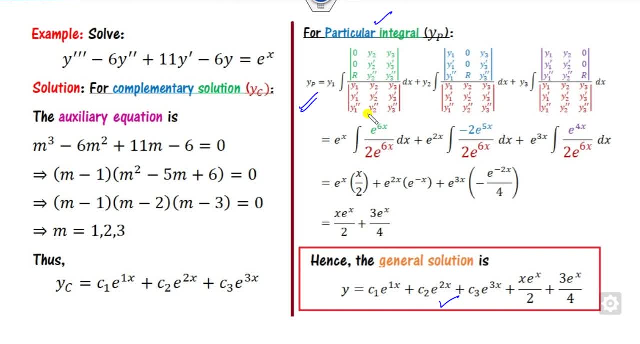 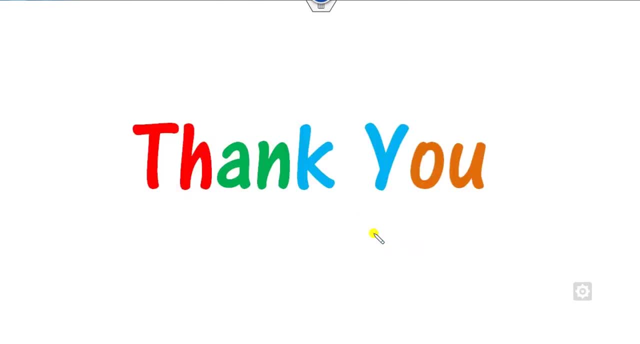 remember. these are there. that will beneficial for you. we will see in our next class some more lectures on the differential equation. till then, you can simply follow this link for finding the various videos. best of luck to you, students, happy learning. 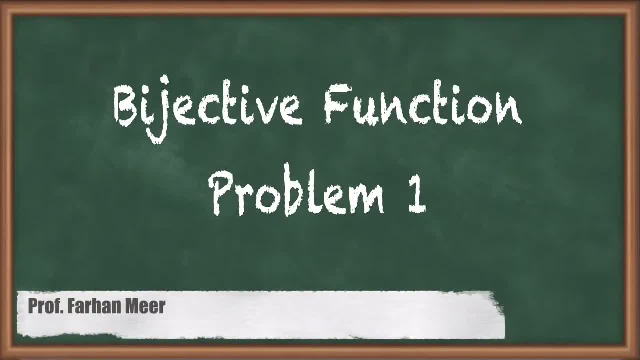 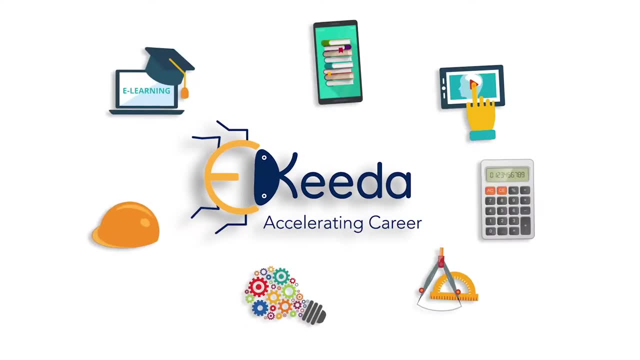 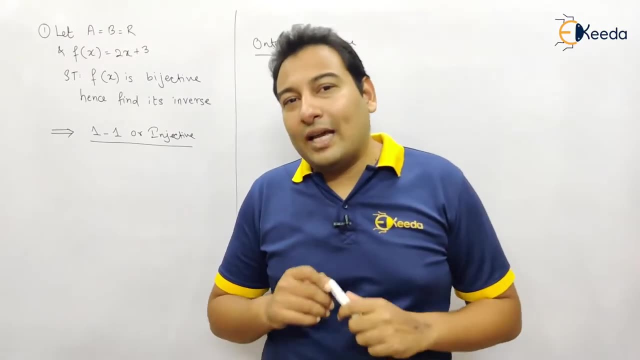 Hello, friends. in this video we'll be discussing problem number one on types of function. Welcome back, friends. Now we're discussing the first problem on types of function. Here we need to prove that the function is bijective and we need to find it inverse. 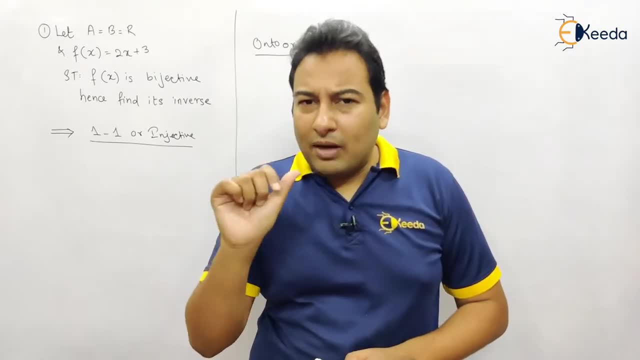 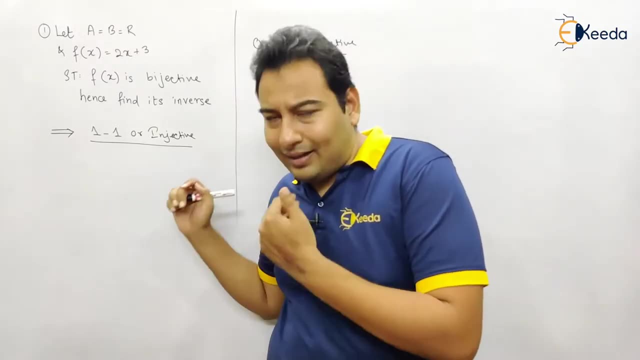 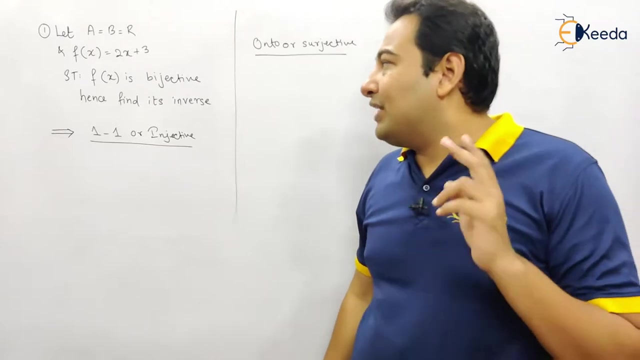 First of all, you need to remember a point: If a function is bijective, then only you can find its inverse. So we'll prove it. It is injective bijective, then we'll find its inverse. So let us start For proving that the function is bijective. two things: we need to prove that.